That's pretty cool. You had quite a few in the 80s and the 90s. So we had four in the 90s: one, two, three, four, five, six, So 10 out of 16,. 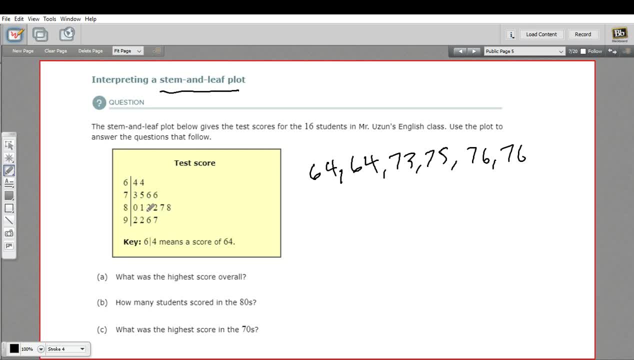 got either 80 or 90 scores on there, So it looks like these students are scoring pretty well. Well, let's see if we can answer these questions now that we kind of understand this group of numbers. A says what was the highest score overall. 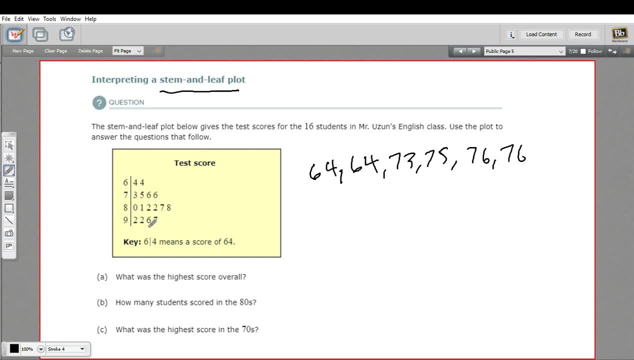 Well, the highest score is gonna be 90 something. So I got down to the nine and then I find the highest number here. that's a seven. So that is 97.. That's the highest overall score. B says how many students scored in the eight. 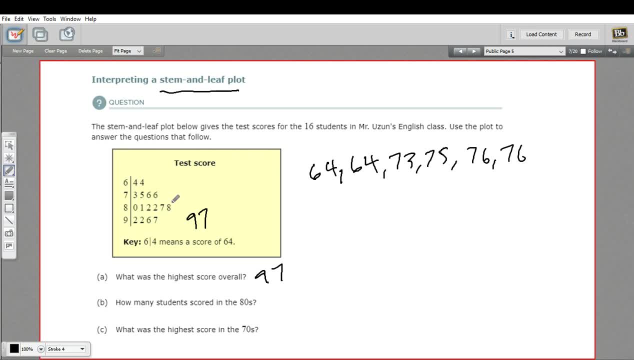 Well, we've got an 80,, an 81, two 82s, an 87 and an 88.. That's one, two, three, four, five, six. Just count the numbers here, That'll tell you how many 80s there were. 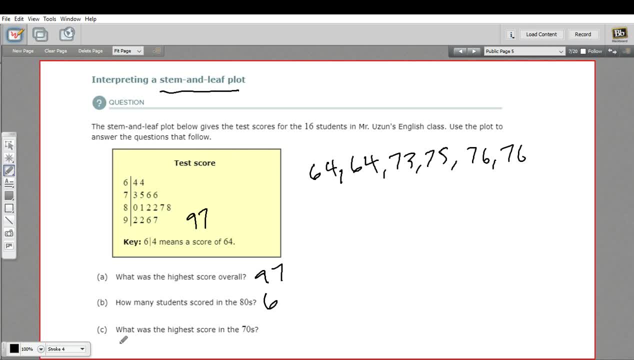 So that's six students who scored in the 80s. The last question C says what was the highest score in the 70s. Well, here are the 70s. I can just go to the end, and that would be a 76.. 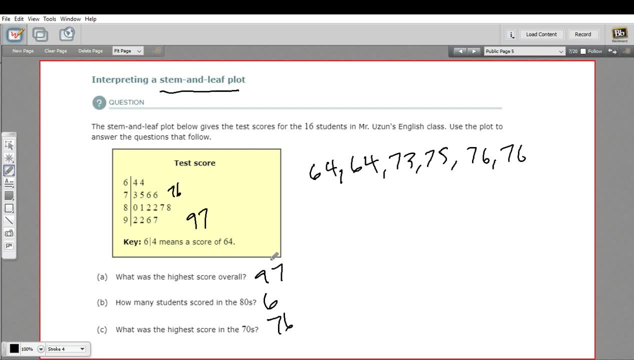 So a 76 is the highest score in the 70s And that is a little bit of work with interpreting- interpreting a stem and leaf plot. 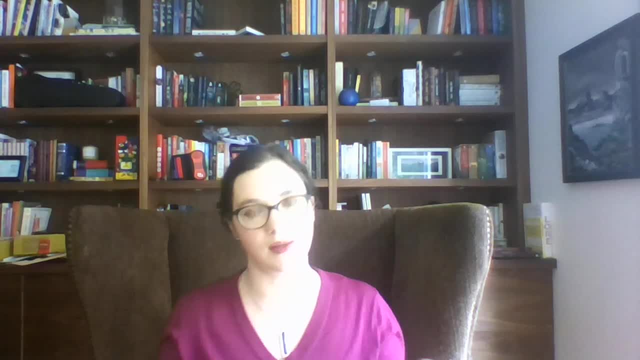 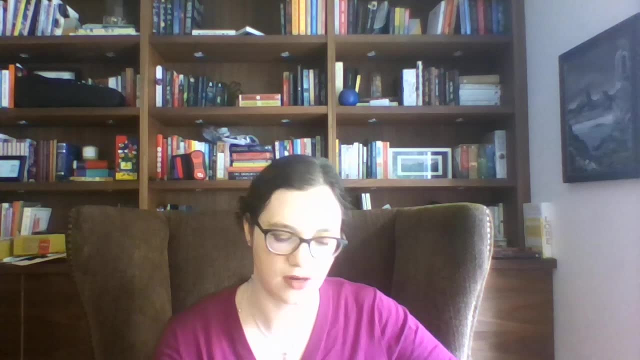 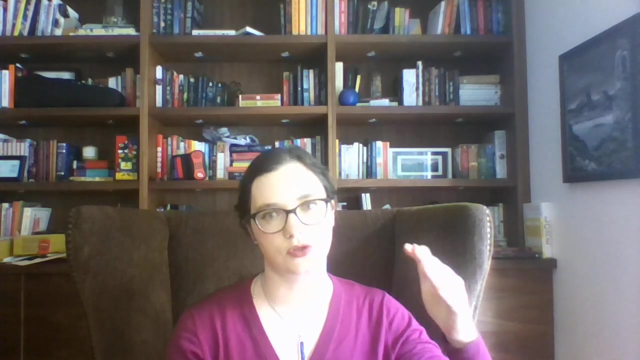 Okay, so this video all about social mobility. It's all about how we move from one position to another, And we're going to talk a little bit about sort of classifying class positions next. but for right now we're going to talk about social mobility sort of in a broad sense, and then we're going to talk about how we understand systems of stratification.